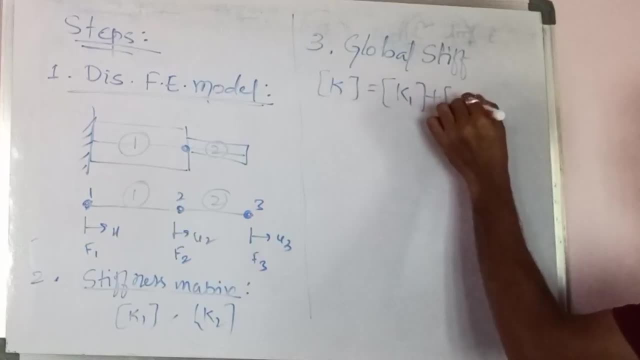 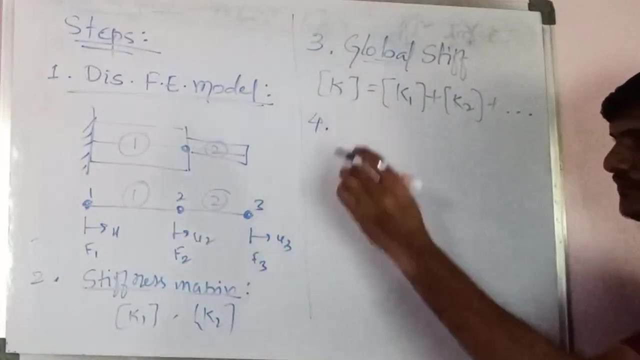 matrix where k is equal to k1 plus k2 plus k3, or if you have another elements you can add now, okay. so using the methodology of the global stiffness method, you have to apply and you have to calculate the global stiffness matrix. and the fourth one, fourth step, it will be: 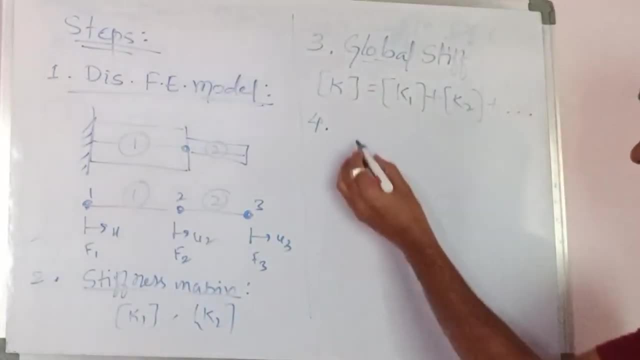 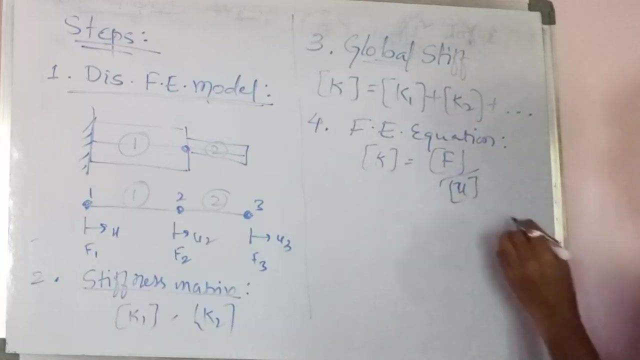 making the formation. okay, formation of finite element equation. so you have to make the formation. so what is the formation? where stiffness matrix is equal to force per unit area, so k is equal to force per unit area, sorry, force per unit deformation. or where k? u is equal to f. 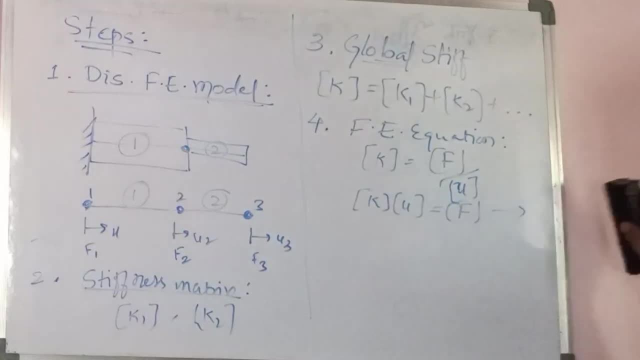 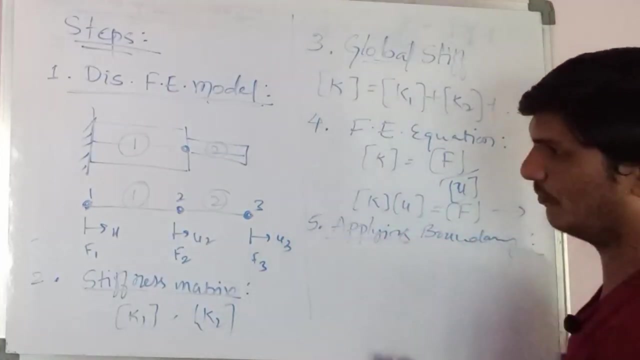 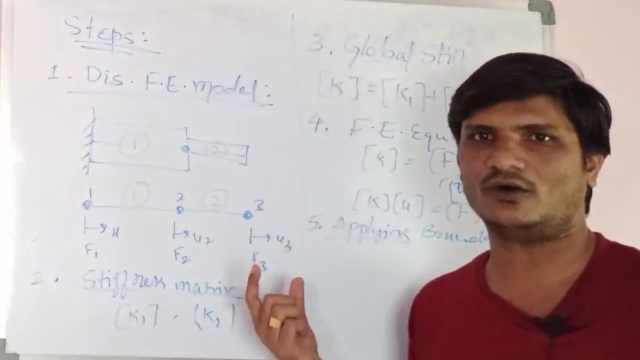 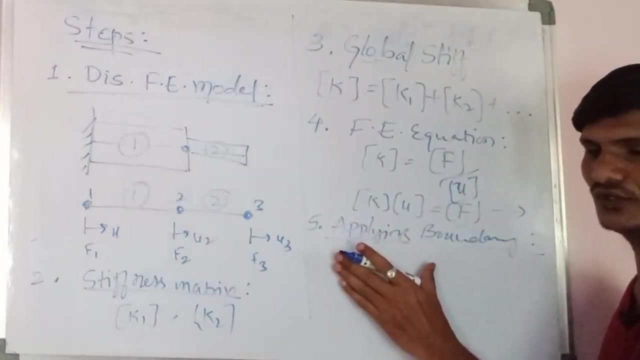 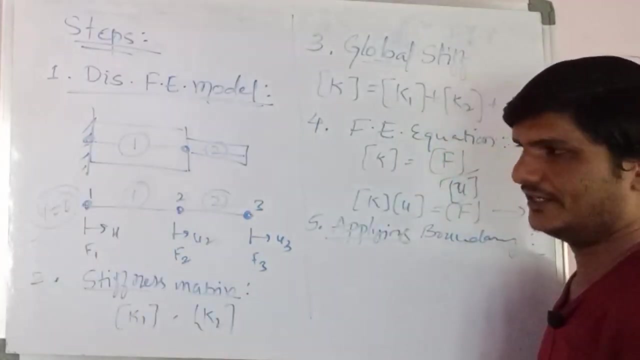 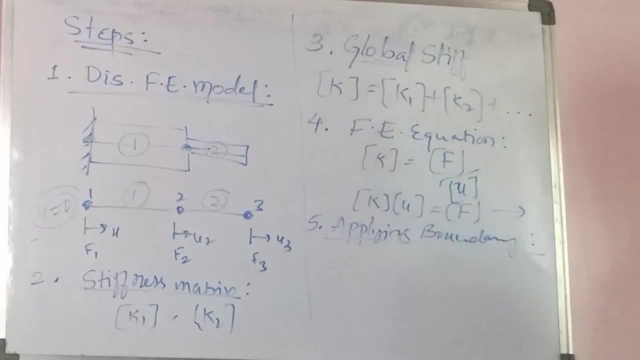 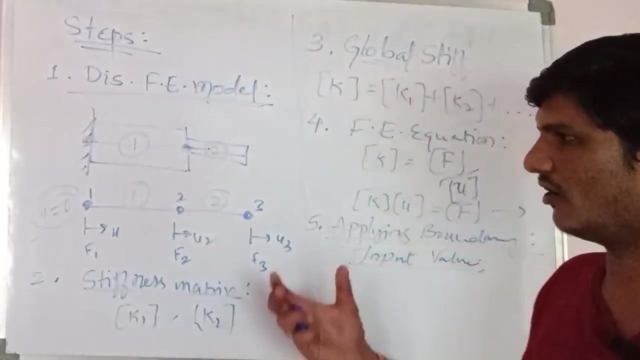 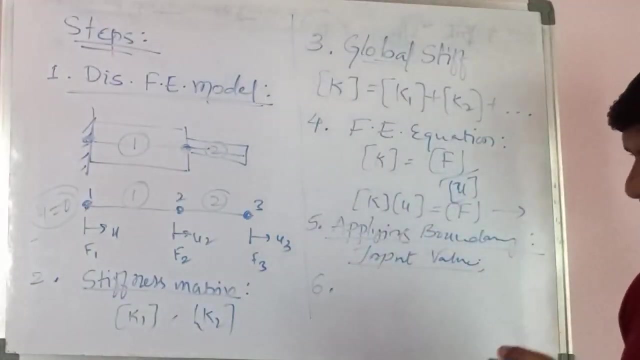 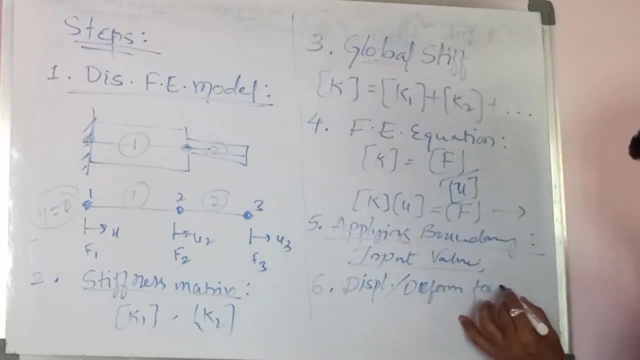 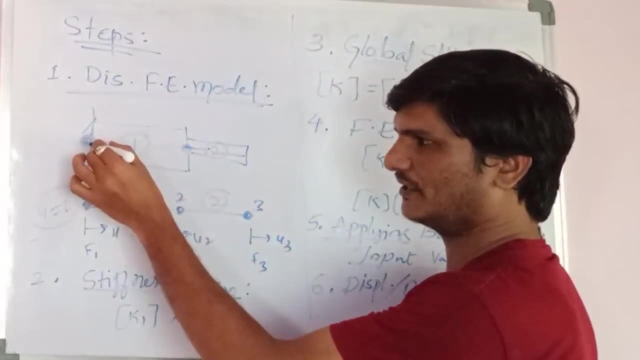 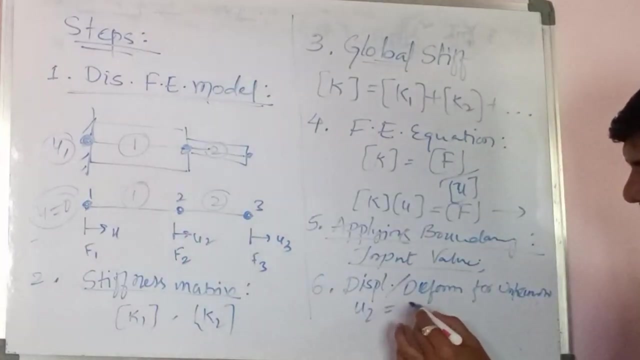 for unknown values. okay, so now where here, in this particular case, u1, it will be 0, so u2, u3, you have to calculate. okay, so that is the unknown displacement. u2, u3 are the displacement you have to calculate. okay, so after calculating, after calculating the displacements or deformation, 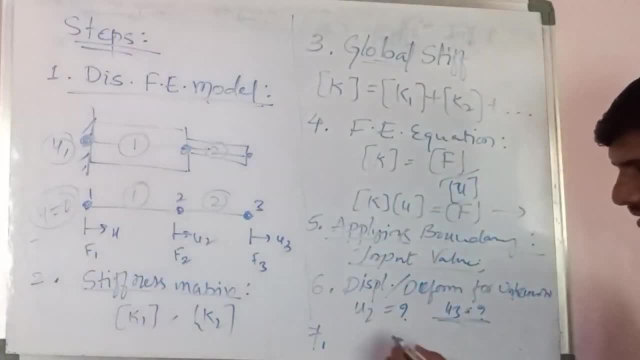 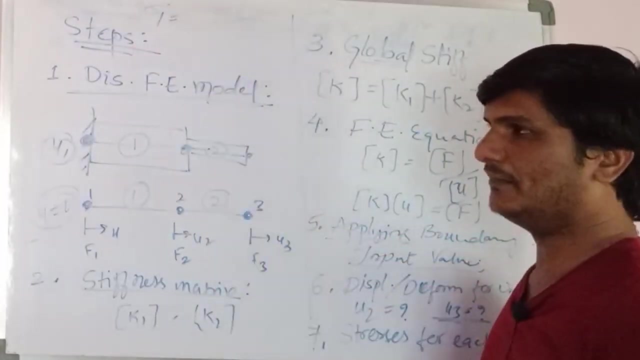 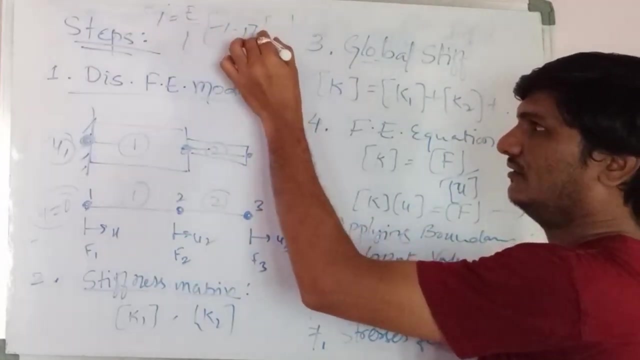 you need to calculate the stresses. okay, stresses for each element. so there are two elements, element 1 and element 2. so stresses is nothing but sigma 1. for the bar element, it is e by l minus 1, 1. so here displacement, that is u1 and u2. so this is a equation for the bar element. 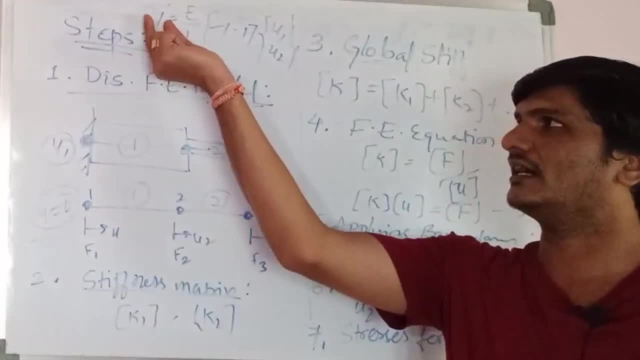 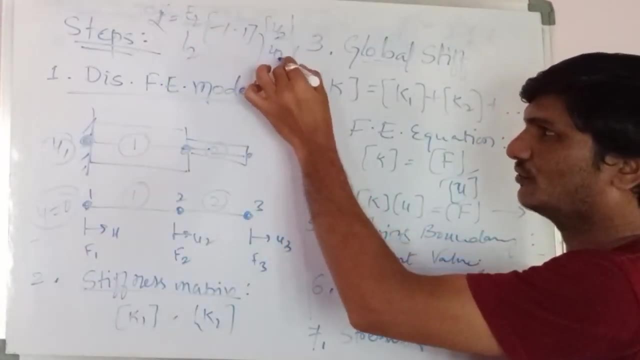 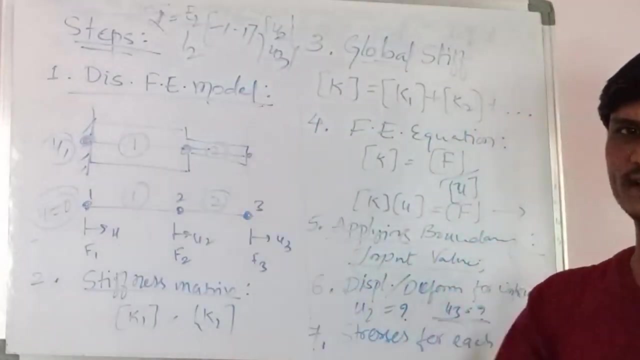 so using this equation, you have to calculate the stiffness matrix for element 1. so now, if you are calculating for element 2, there will be sigma 2, e2, l2 here, u2, u3. so based on that you have to calculate the stiffness- sorry stresses- for the individual element. 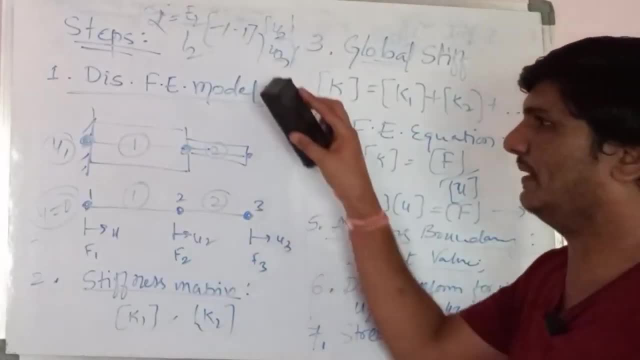 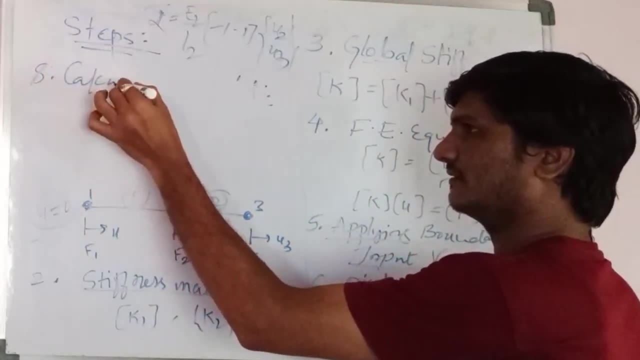 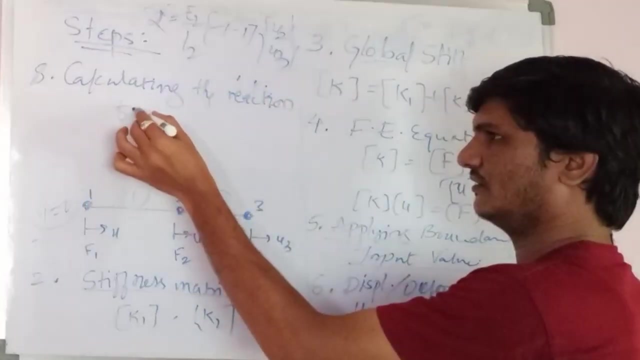 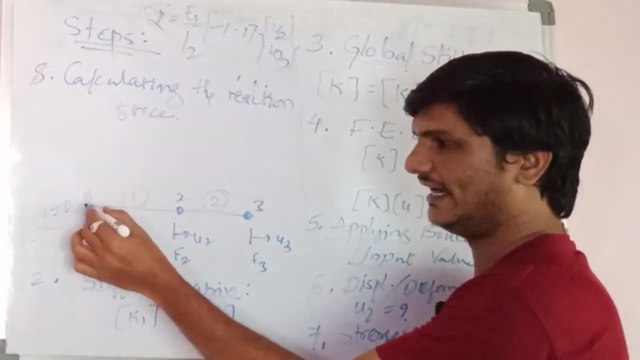 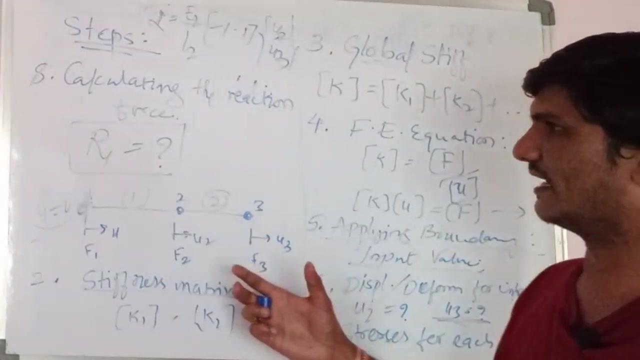 so once you calculated the stresses, then the last step it will be to calculate the reaction forces at 1. calculating the reaction forces, okay, for the given problem. where the node one is fixed, it means there is a reaction force at node one. it means r1. you have to calculate, okay. so like that, these are the around eight to. 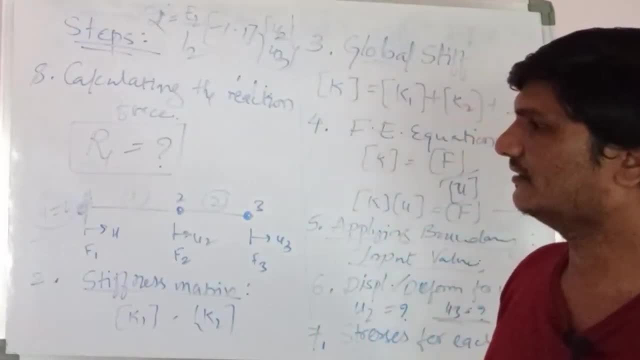 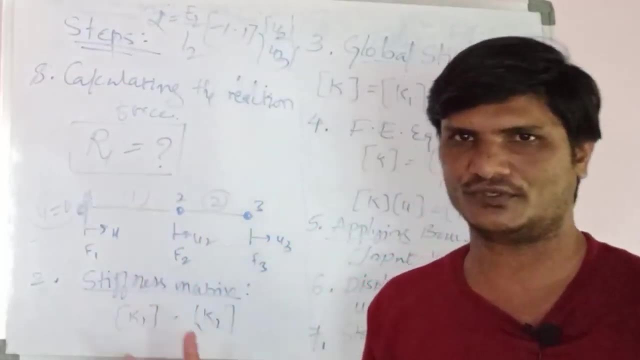 nine steps in the finite element method. you have to determine the first displacement and you have to determine the stresses and also you have to determine the reaction forces. so these are the basic steps in the finite elements method. so thank you for watching.